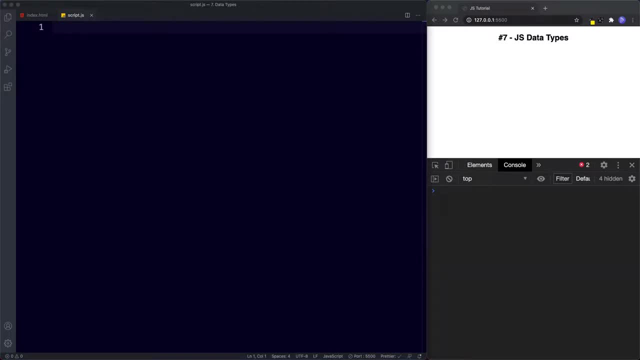 always of a certain type. These types are known as data types. For example, in the previous lessons you've seen me type something like this. So we can say: let num be assigned the value of seven. Here we've assigned the value of seven to our 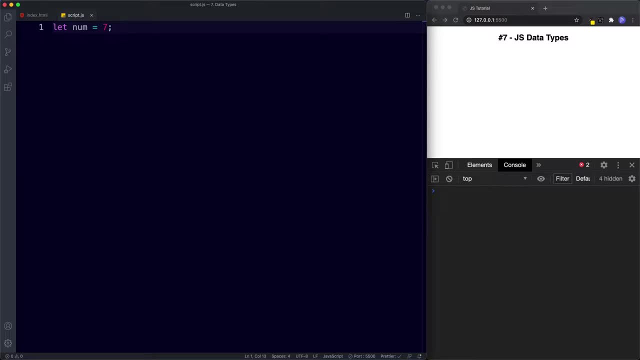 num variable. This is known as a number, data type or simply a number. We can also say something like: let channel be assigned the value of dev dreamer. So here, the value that we've assigned to the variable named channel is dev dreamer. This particular value is known as a. 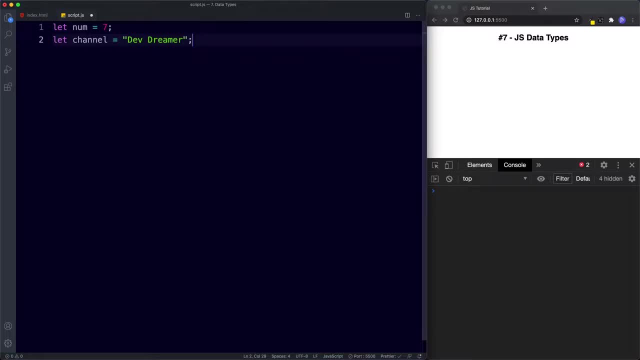 string. This is a string data type. Notice the quotation marks thrown in the words. So, as you can see, JavaScript contains different data types and is more than just numbers and strings. Let's now take a look at the different data types that we have available to us in JavaScript. Okay, so the best way to think, 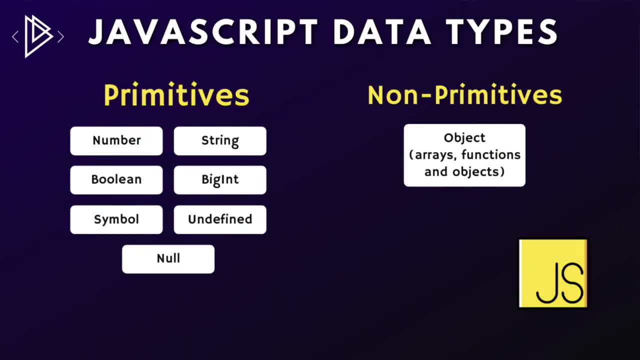 about these data types, then, is in terms of primitives and non-primitives. It's always good when we can categorize things, makes things easier to learn. So first let's take a look at the primitive data types. So we have number string. 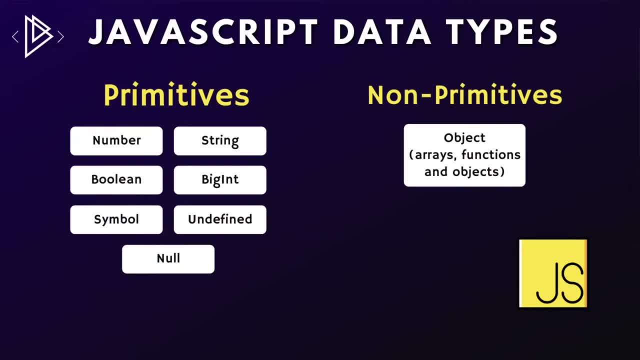 boolean, big int and string Symbol, undefined and null, So these are all known as primitive data types, or simply primitives. For non-primitives, there's only a single data type called object, and these could be things such as arrays, functions and objects themselves. 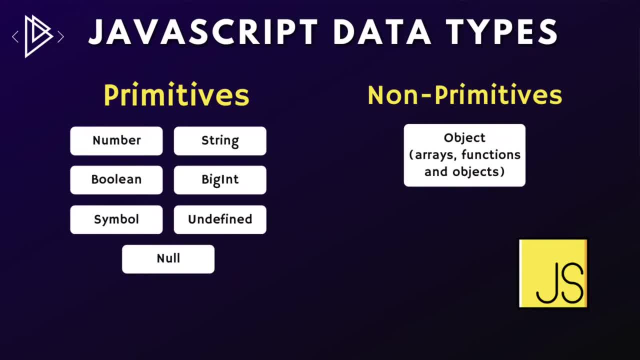 Don't worry too much at this stage if that confuses you. Everything will be made clear as we progress. So, as mentioned then, these first seven are known as primitive data types or simply primitives. The word primitive means simple or basic. Now, the reason why these are known as primitives is because the 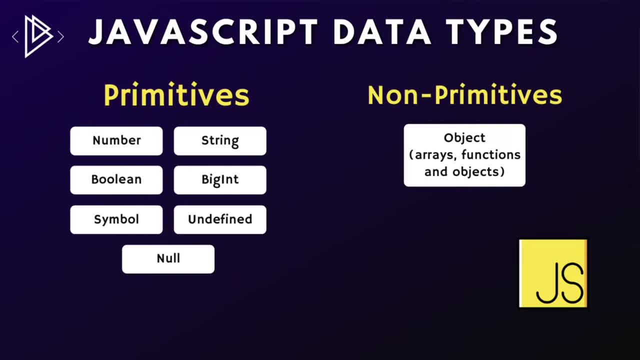 primitives hold- remember we're looking at data types in this lesson- are single, simple data values. Those values are immutable, meaning that we cannot change those values and those values have no properties or methods. Now, at this stage, that might confuse you because you might be saying: well, what are properties and 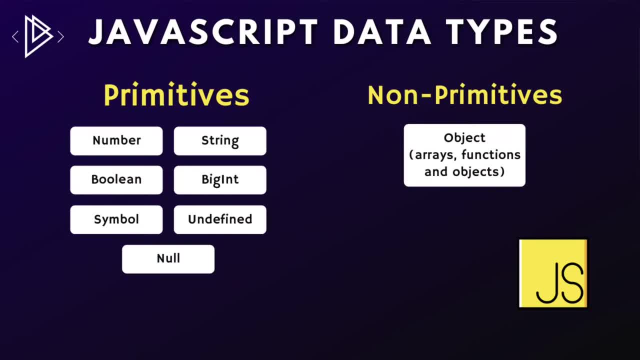 methods anyway. and that brings me nicely on to the object data type. Remember, we said that primitives can only hold single, simple data values. Well, in contrast, an object data type is used to store multiple and more complex values. Now what we'll do as we go throughout this. 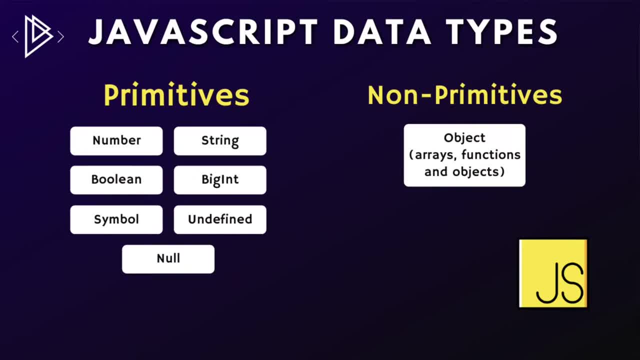 series is. we'll deal with these primitive types first, and then we'll start looking at object data types in detail, So arrays, functions and objects themselves- And, by the way, objects are a huge part of JavaScript, as you'll come to see. So think of this lesson then as an intro to the different data types. 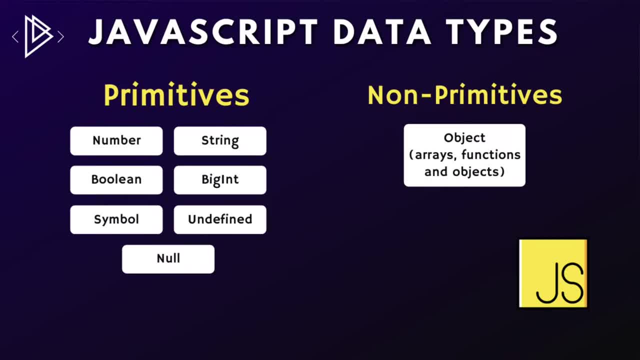 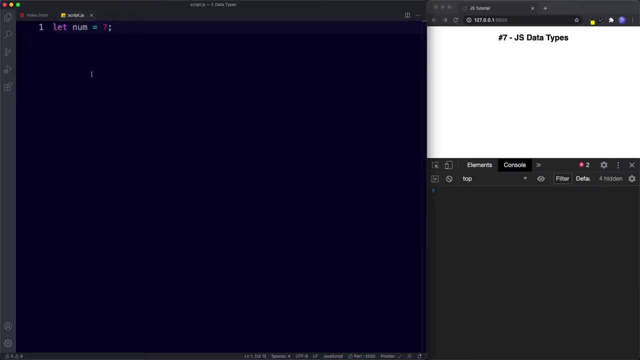 Let's start, then, with looking at the primitives. first We'll start with number. Okay, so first let's go ahead and remove this string. So we've just got our number data type now. So, unlike some of the languages, JavaScript has only one kind. 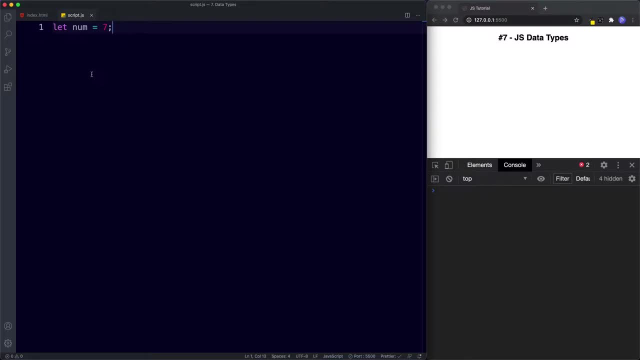 of numerical data type for whole numbers and decimals, Simply called number. Other languages might use int, which is short for integer for whole numbers and then float for decimal numbers, but in JavaScript the number data type can handle both. So, for example, we can say something like let: 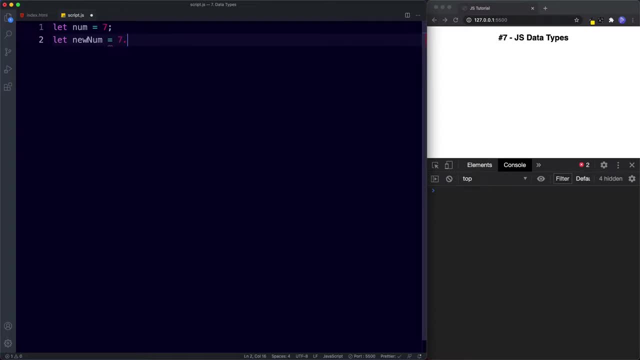 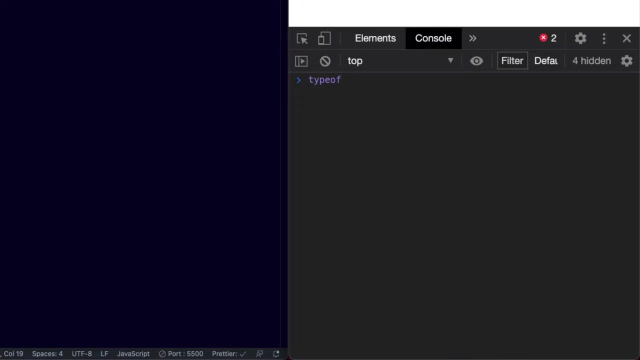 new num be signed, the value of 7.58.. So these are both known as numbers. Now JavaScript actually gives us a built-in keyword called type of and that basically is used to identify the type of a variable. So for example, down here in the console I can say type of space and then the number. 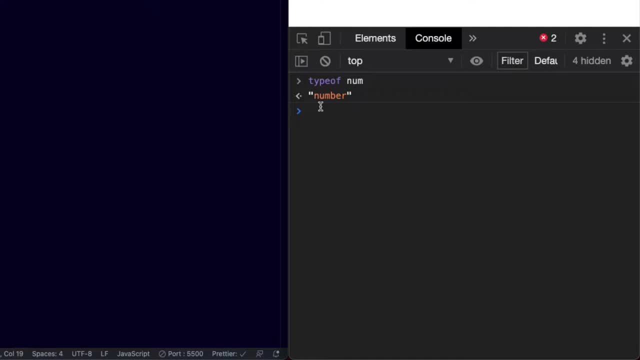 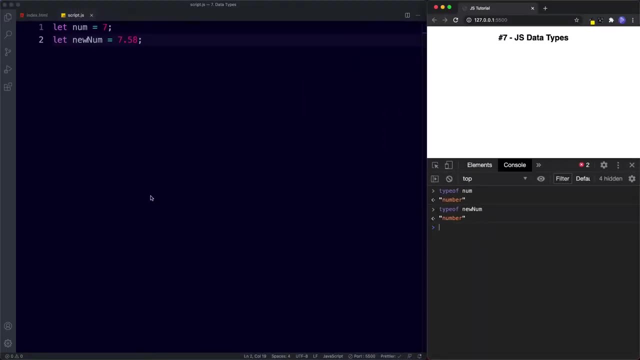 num variable, press return and here you see, it returns number. we can do the same for the other variable so we can say type of that was called new num and again it returns a number. we're going to be looking at numbers in a lot more detail later. on the next primitive data type we want to look 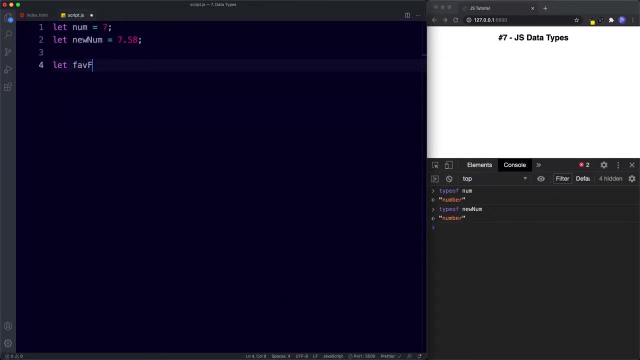 at is strings. so we can say something like: let fave food be assigned the value of pizza and let fave color be assigned the value of purple. now, a string is always surrounded by quotes. these quotes can be double quotes, as we've got here for pizza, or single quotes, as we're using here, so strings. 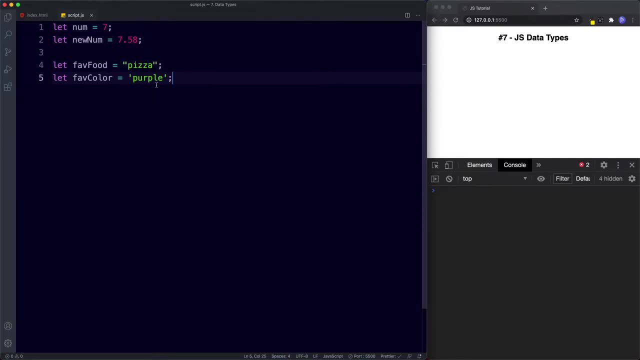 are basically text values, whether it's a single letter or an entire paragraph, because we're working with text. it's going to be a string data type. we'll look at strings in a lot more detail later on. okay, the next data type we're going to look at is the boolean data type. now, the boolean data type. 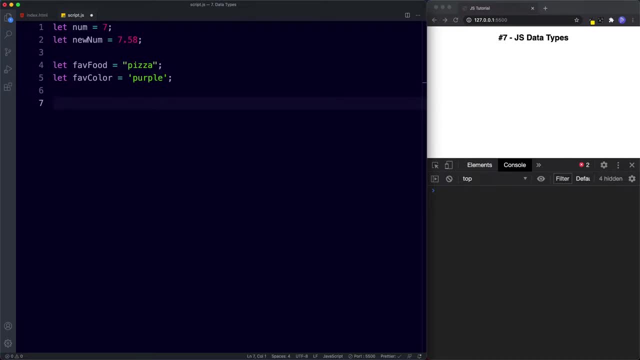 has only two values- it can either be true or false- and this might give you some indication as to what booleans are used for. they can be used to compare and assess a condition and then perform an analysis of the data type, and then perform an analysis of the data type and then perform an. 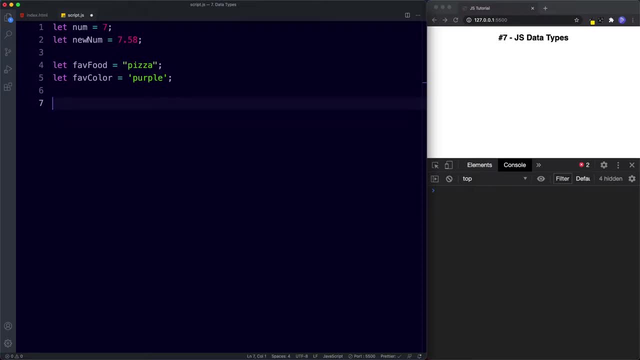 action, depending on whether that outcome is true or false. we'll look at booleans in more detail later on. for now, let's take a look at a quick example. so here i'm just going to say consolelog and in the parentheses here i'm going to say 1 space greater than 100.. now, if you save this and have a look at, 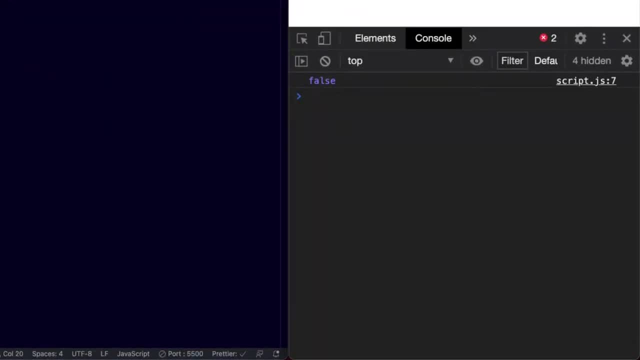 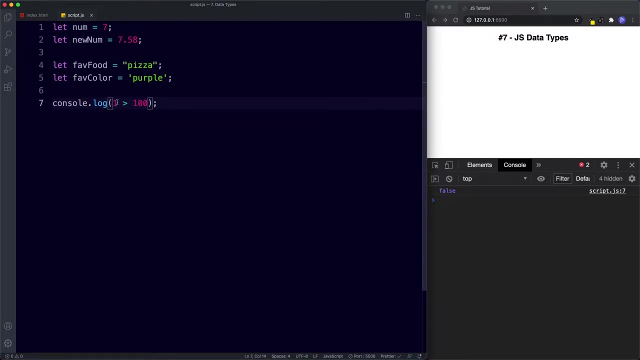 the console. the console returns false and that's because this isn't true, right? this condition is not true. 1 is not more than 100, so this is false. if we said: is 100 more than 1, then this will return true, because 100 is. 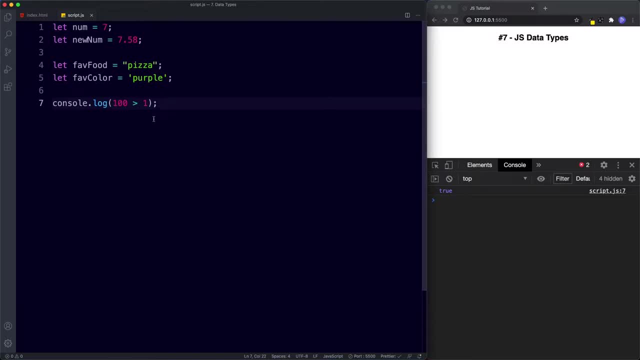 more than 1. you'll see the advantage of this as we progress through the series. let's take a look at another example. we could say: let js be assigned the value of string, which is cool, and then down here let's log js double equals cool, and you might remember that in a previous lesson we spoke about. 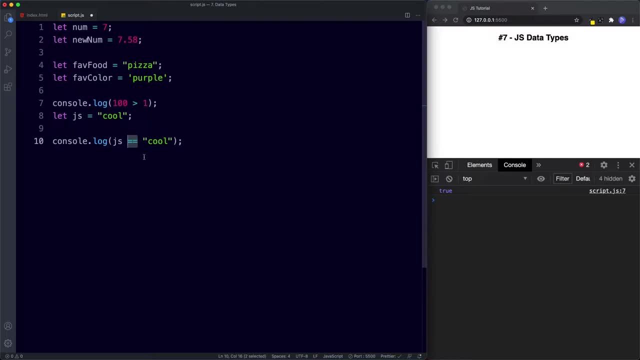 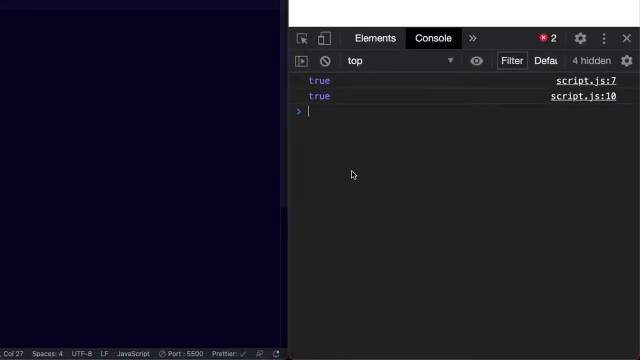 the fact that javascript uses this double equal symbol here to compare two values to see if they are equal. okay, the single equal sign, remember, is used to assign values. so what we're checking here is we're checking to see if javascript, the variable javascript, ень Blessed. once again, we get true in the console, and of course, we'll look at booleans in a lot more. 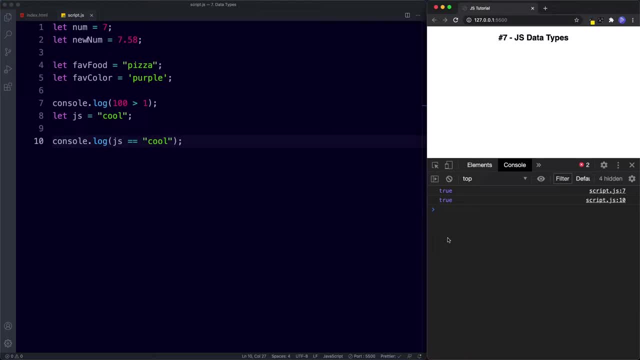 detail later on. okay, the next primitive data type is big int. the bigint type was created to handle really big numbers. the number data type cannot represent a number bigger than. i'm not going to say this, i'm just going to type this out. and if we use type of to 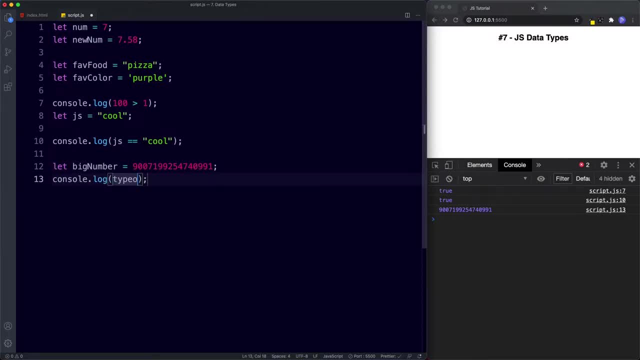 check the data type of big number. let's see what we get back. so let's do console log typeof big number. okay, the consolelog typeof Console returns number to us. so the BigInt data type and Integer, short for Integer, was used to handle numbers that are bigger than this. 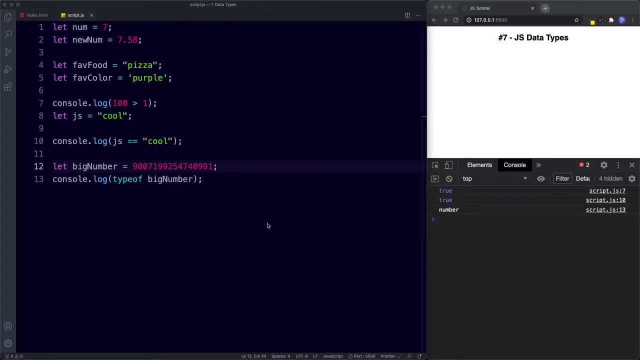 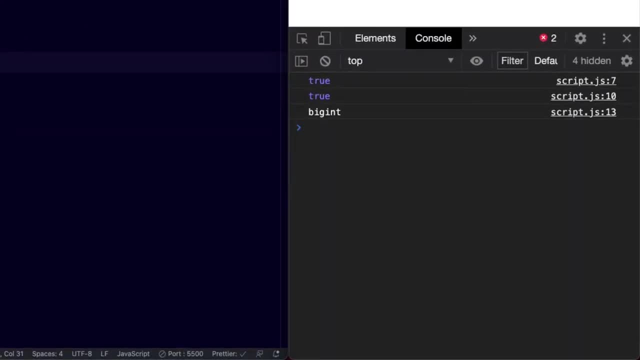 Now the way that we declare something as a BigInt data type. we simply add the letter N to the end. So if we come here, let's change this to 2, add the letter N, save this and now we can see. the type of BigNumber is now BigInt. 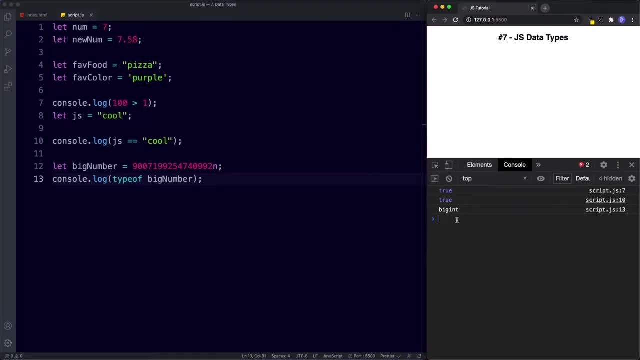 Now chances are it's going to be quite rare that you're going to be working with really, really big numbers like this, so for now, this explanation will suffice. The next data type symbol can be created by invoking the symbol function, and it's basically used to create unique identifiers for objects. we'll look at symbols when we cover objects. 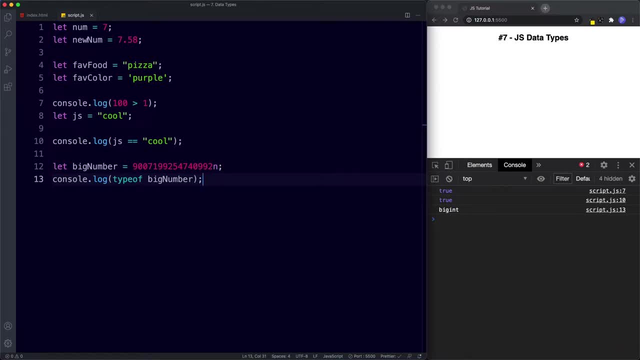 in detail in a future lesson. Okay, the next data type is undefined. now, undefined is simply a variable that has not been assigned a value. So down here, let's say let channel name and then just end it with a semicolon. So here, remember, we've declared this variable, but we haven't initialised it with a value. 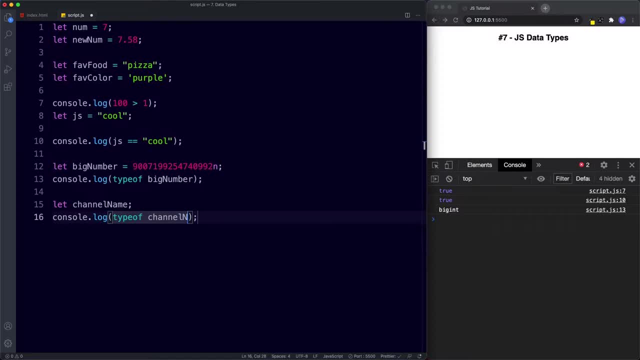 If we now log the type of this variable, you can see that the console returns undefined. and it makes sense. the clue is in the word right- undefined. whilst we've declared this variable by saying let channel name, we haven't actually assigned a value. 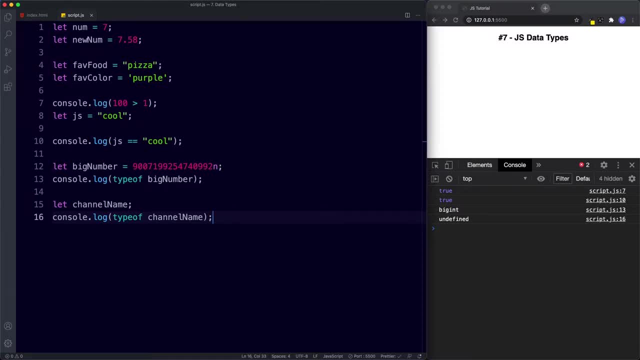 to this. we haven't actually defined this variable. Okay, and now the last data type is null. now, there's sometimes some confusion about the difference between undefined and null. they're different as to their type. Null is used to declare a value as empty, so null is something that we specifically 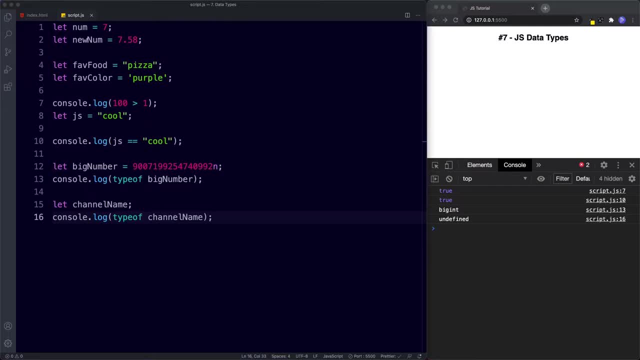 declare a value as, whereas undefined, is reserved as the default data type for variables that have not been initialised, Like this channel name variable here. Okay, so that's all of the primitive data types. let's now take a look at our single non-primitive 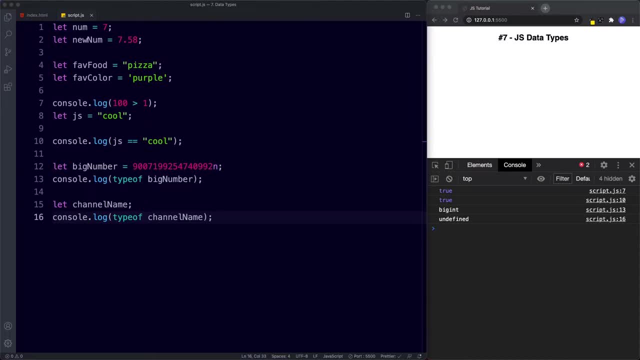 data type called object. So, as mentioned earlier, then object data types are used to store multiple and more complex values. An object data type can be an array, a function or an object. Let's take a brief look at each of these now, and of course we'll be looking at these in. 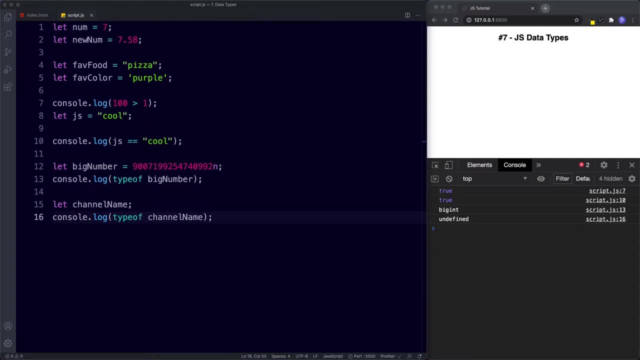 more detail as we progress through the series. Let's start with arrays. Remember we said that primitives can only hold single data values, whereas objects can hold multiple values. Well, an array is basically a list of different values. So to create an array, we simply say let and then create your variable. so I'm going to 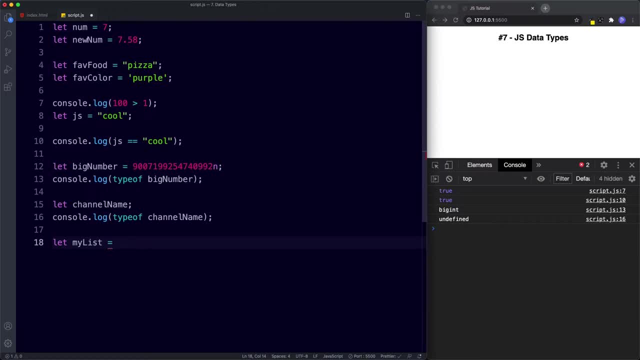 call this my list. We assign the value, and then now to create an array in javascript, we simply type square brackets like so: And now inside these square brackets, we can start listing out some values. So I'm going to say amit, and these are all going to be comma separated. 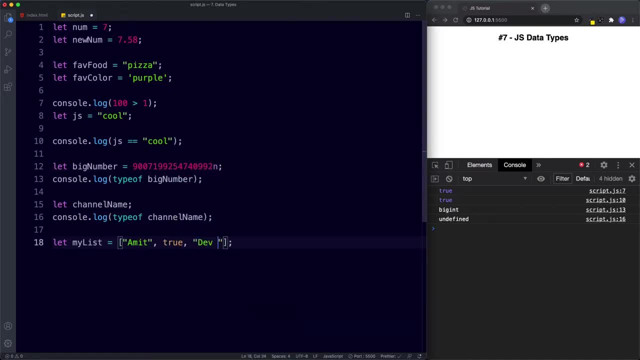 Let's go for a boolean value, so let's just say true. let's say dev dreamer, and let's also put a number in here as well, so let's just say the number seven. And now, if we consolelog this In the console, here we get this parenthesis with four. okay, because this array contains: 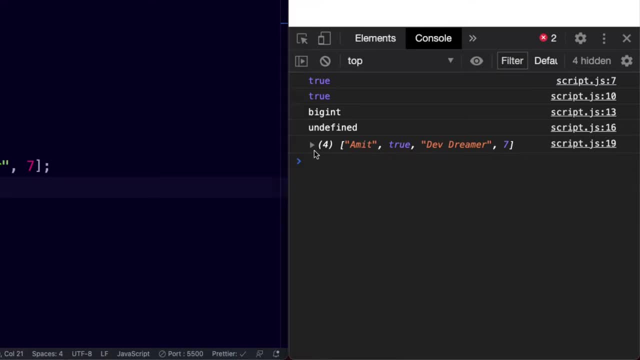 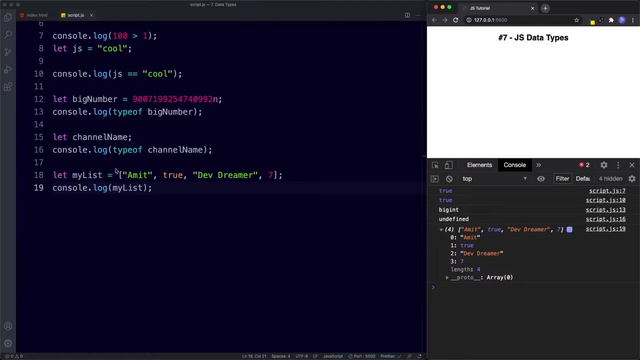 four items: one, two, three and four, and we can also expand this as well, and that gives us a bit more information about this array. To access values within the array, we simply type out the name of the array, which is my list, and then at the end here we do square brackets and then inside, here we're going. 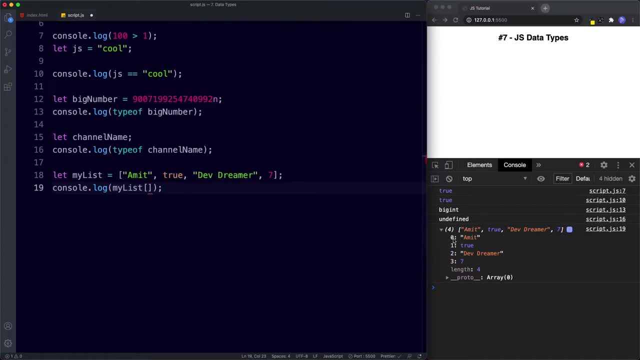 to type in a number Now the number that we're looking for is basically these numbers here, so zero, one, two and three. So, for example, if I said the number one in here and save, you can see we get the value. true. if I said two, we get the value. dev dreamer. 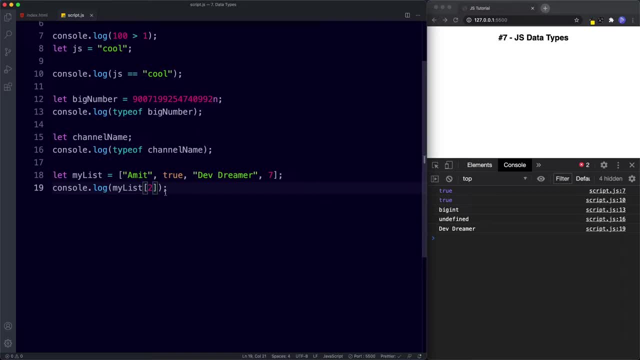 So to access values inside an array, we use the square brackets and then a corresponding number. Now you might be thinking: why is dev dreamer assigned the number two when actually it's in the one, two, three, the third position? and in fact, why is it that when we type in three, 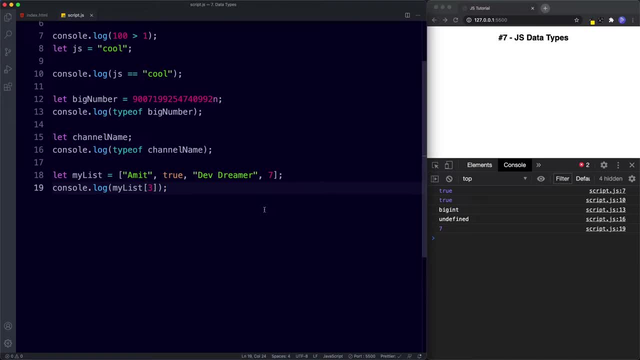 we get this value, the number seven? well, that's because arrays are zero indexed, meaning the first value is always zero, and then it goes one, two, three and so on. We'll look at arrays in a lot more detail as we progress through. Okay, next up we have functions. so a function is another object data type. so to create a 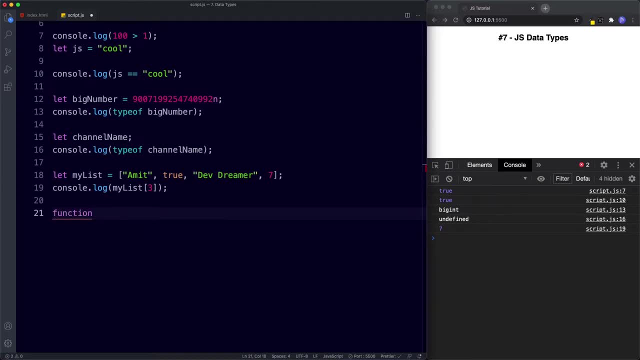 function, then we can just say the word function space, and I'm going to call this function hello, and then do a parenthesis after it, curly braces, and then inside these curly braces is basically going to be our code that we want to run. So I'm just going to say console dot log, hello. and then down here outside of the curly braces, 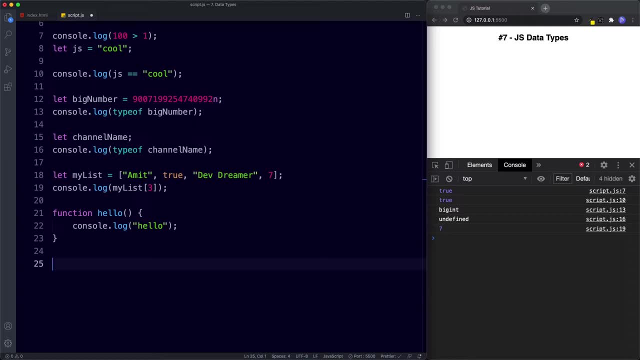 I'm going to call or invoke this function by using the function name, which was hello, and then the parentheses, And just let you know, it's actually the parentheses that is responsible for invoking this function. So let's save and in the console here we get the word hello and we can use this as many. 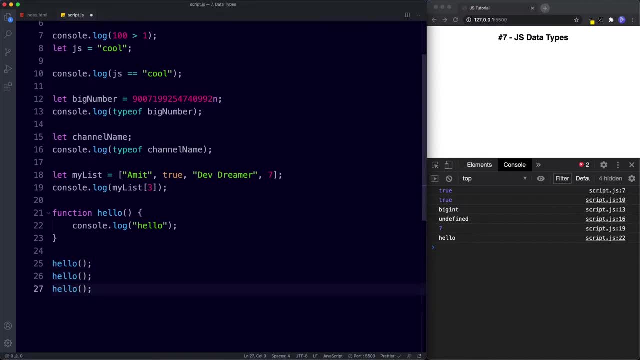 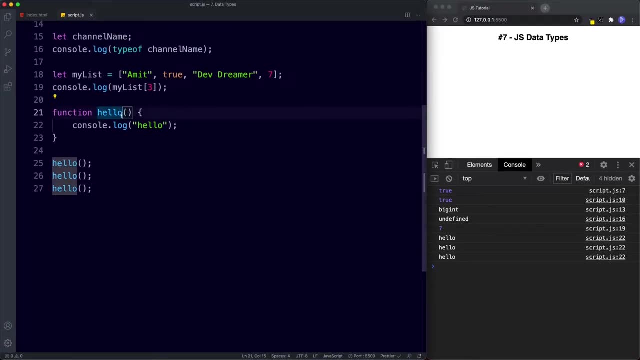 times as we like. so we can say again: And in the console we get hello three times. Now we can also assign this function to a variable name. So for example, let's just remove the function name from there, Let hello be assigned the value of function. 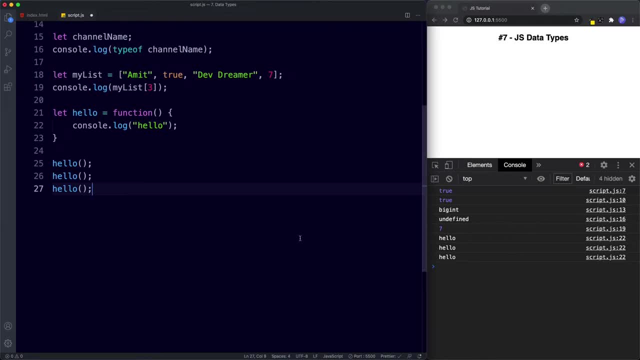 And if you save this, as you can see, that still works. Once again, We'll look at functions in a lot more detail later on. Finally, let's take a look at objects again. objects can be used to store multiple values. Let's take a look at an example. 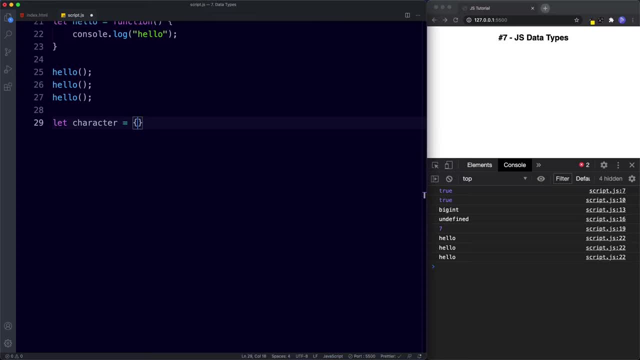 So here I'm going to say: let character be assigned the value, and then to create an object, we do curly braces like this, and then inside these curly braces, objects basically contain name value pairs. So I'm going to say: name colon space and let's assign this a value of Sonic the Hedgehog. 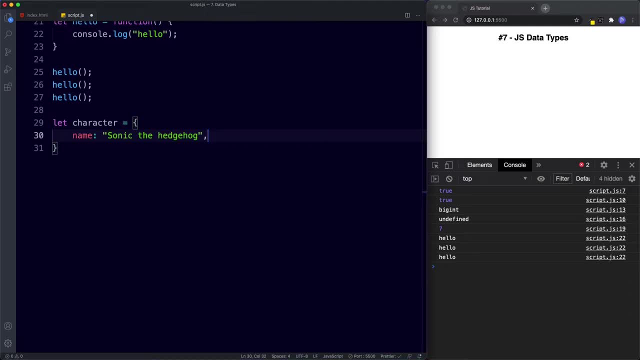 and then we say comma, So these name value pairs will all be comma separated And, just like with arrays, we can actually pull the information out of this, of course. So let's do console dot log, and the way that we do this is we use the object name, which 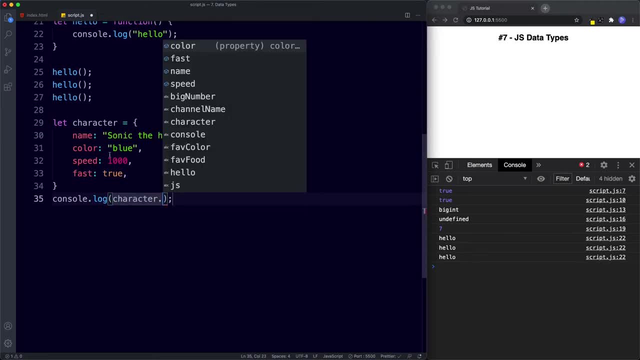 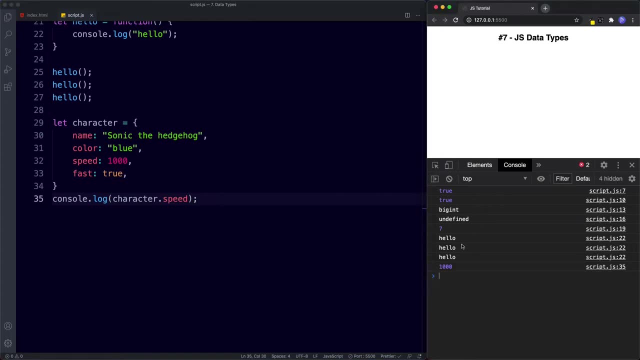 is character, and then we say dot. So let's say we wanted to log the speed, so we can just choose speed. Let's save this and down here, sure enough, we get the number 1000.. So objects then store name, value, pairs and of course we'll be learning all about JavaScript. 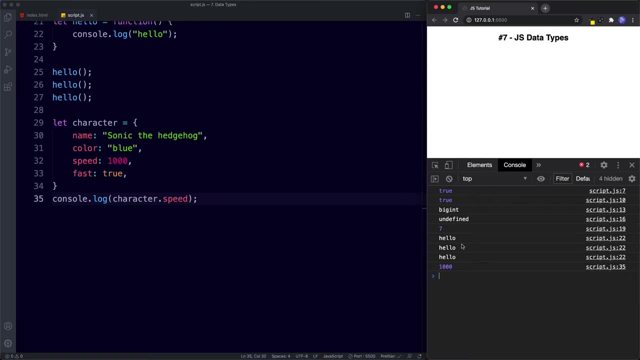 objects later on. To summarize, then, Data types. There are different values that we can use in JavaScript. There are seven primitive data types, and then there's a single non primitive data type called object. Primitives hold single, simple data values, whereas objects hold multiple and even complex. 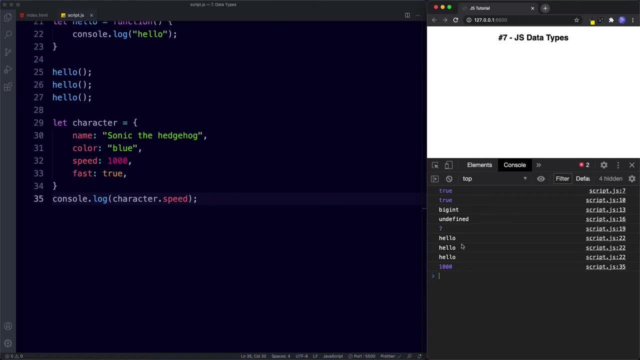 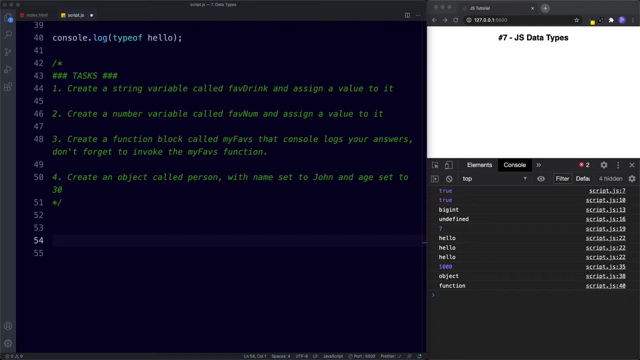 values. Okay, so before we end, then let's take a look at your tasks. So we have four tasks for this lesson. For the first task, I want you to create a string variable called fav- drink and then assign a value to it. For task two, I want you to create a number variable called fav num and assign a value. 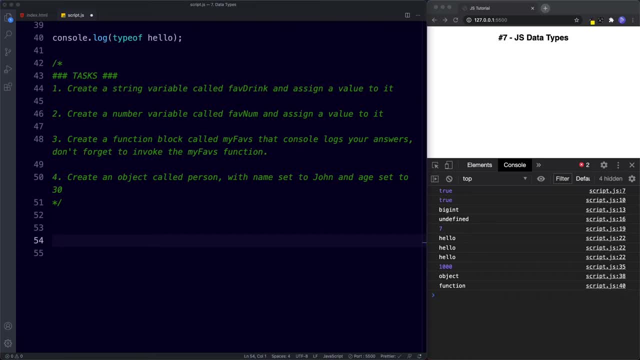 to it. Then, for task three, Create a function block called my favs And then console log your answers from task one and task two. Don't forget to invoke the my favs function. And then, finally, for task four, I want you to create an object called person. 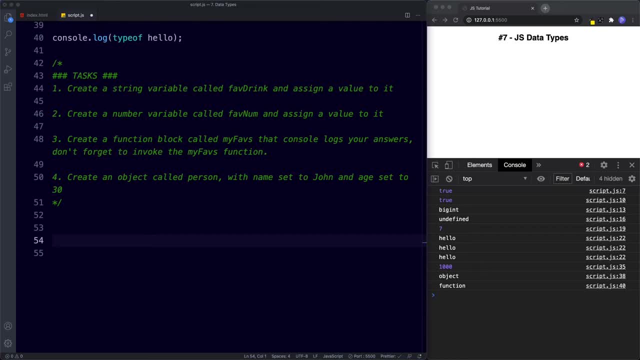 And then inside the object, I want you to set name to john and set age to 30. So go ahead and pause the video and try these out. When we come back we'll take a look at the answers. So how did you get on then?